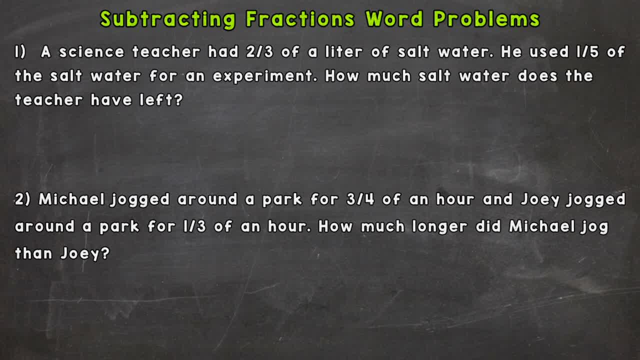 we have a science teacher had two-thirds of a liter of salt water. He used one-fifth of the salt water for an experiment. How much salt water does the teacher have left? Well, in this situation, we're starting with two-thirds and we're using or getting rid of one-fifth, taking away, which is 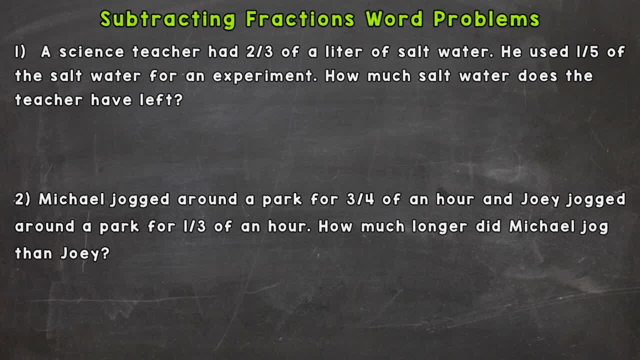 subtraction. So if we're taking something away or finding the difference between the two-thirds, it's going to be subtraction. So again, we start with two-thirds and we subtract or take away one-fifth. So we need to use subtraction in order to get to our answer. So here we don't have a 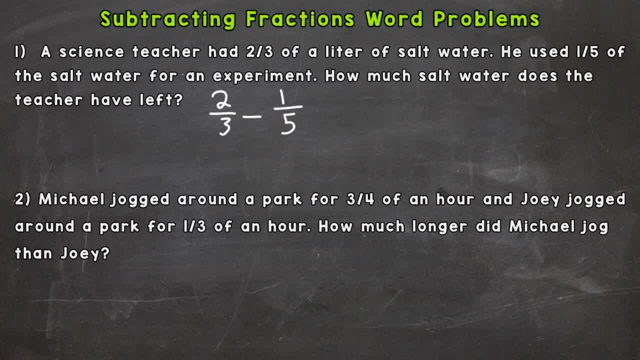 common denominator. So we're going to need to rewrite that problem with the common denominator which for a three and a five. what do you think it's going to be? Hopefully you're thinking fifth. So we're going to need to rewrite that problem with the common denominator. 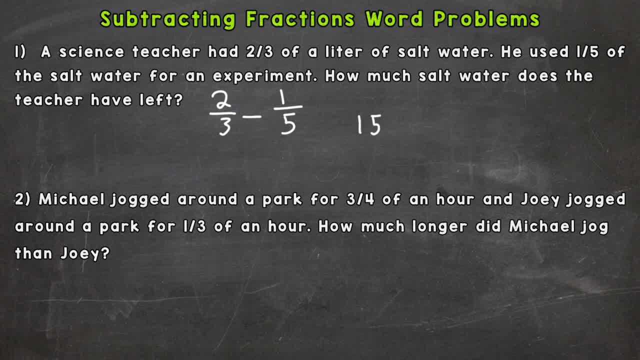 Fifteen. So let's rename with that denominator of 15.. Well, we know, 3 times 5 is 15.. So let's do it to the top to get an equivalent fraction. 2 times 5 is 10.. 5 times 3 gives us the denominator of 15.. 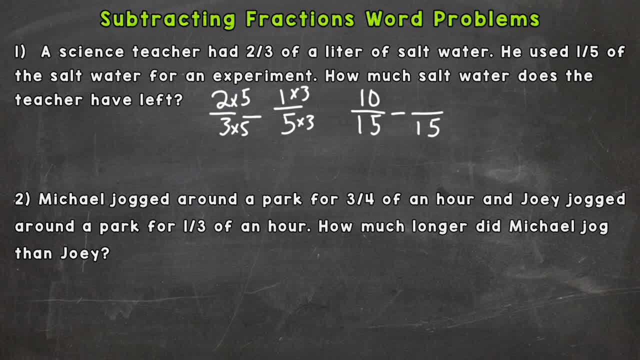 So let's do it to the top to get an equivalent fraction: 1 times 3 is 3.. Now we're ready to subtract: 10 minus 3 is 7. And we keep our denominator of 15 the same. So how much salt. 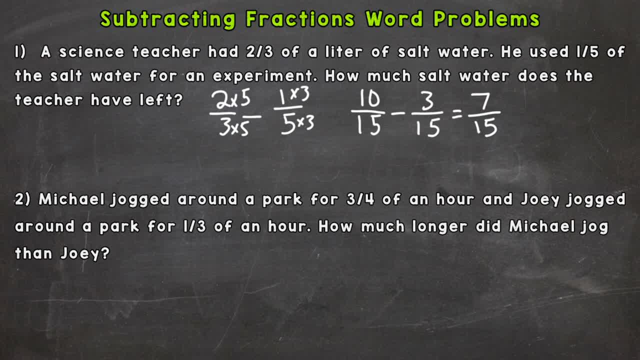 water does the teacher have left? Well, 7, 15ths and this measurement, this is in liters, So 7 15ths of a liter. So again taking something away or subtracting that one-fifth there. So we used a subtraction. Number two: Michael jogged around a park for three-fourths of an hour and Joey jogged 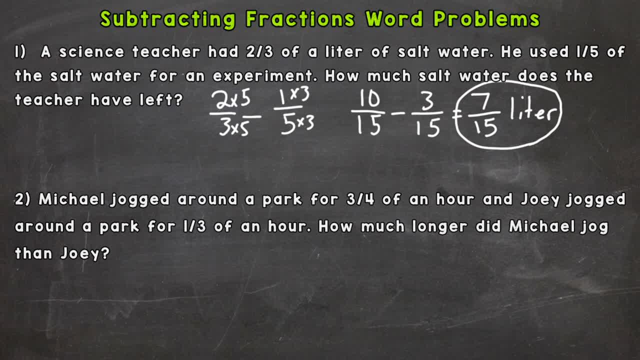 around the park for one-third of an hour. How much longer did Michael jog than Joey? Well, this is a difference problem. We need to find the difference between three-fourths and one-third, or how much longer three-fourths is than one-third. So